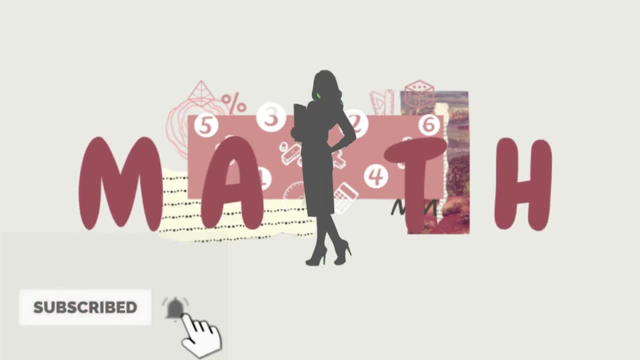 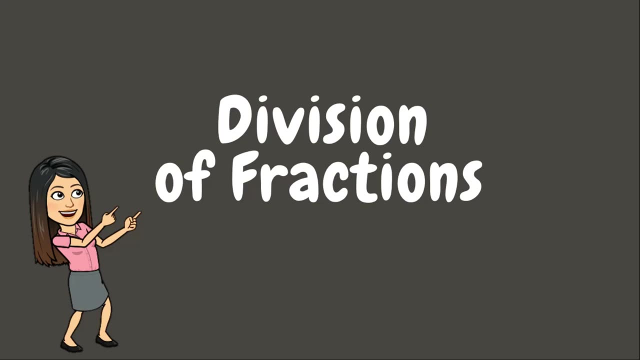 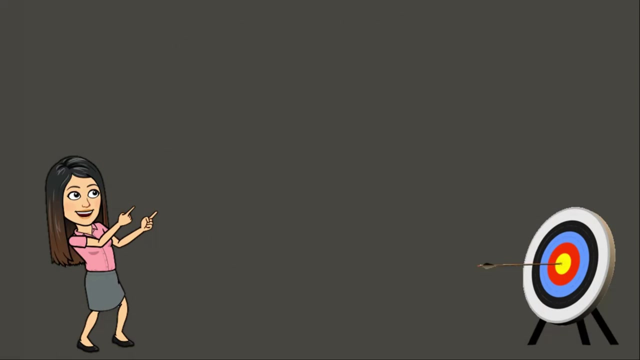 Good day students. Welcome back to my classroom For today's lesson. you will learn how to divide fractions with or without regrouping. Let us begin. Let's try this first example: One-third divided by two-fifths. To divide fractions first. 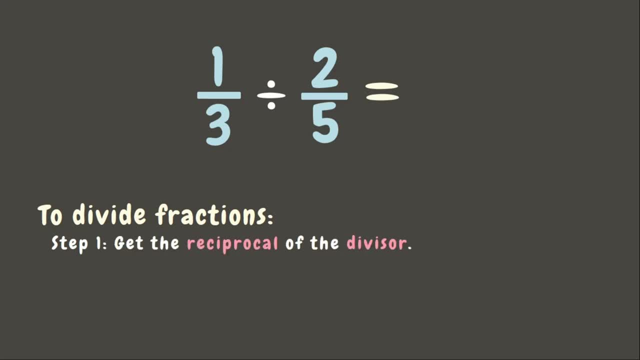 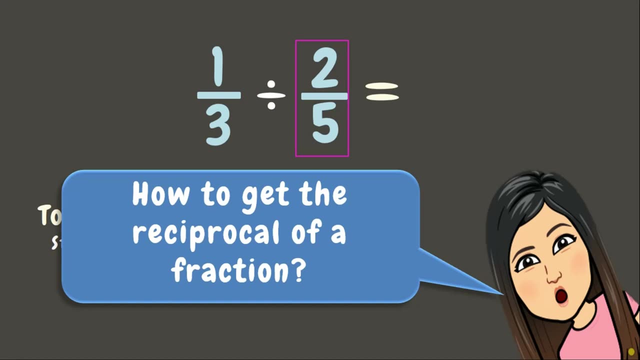 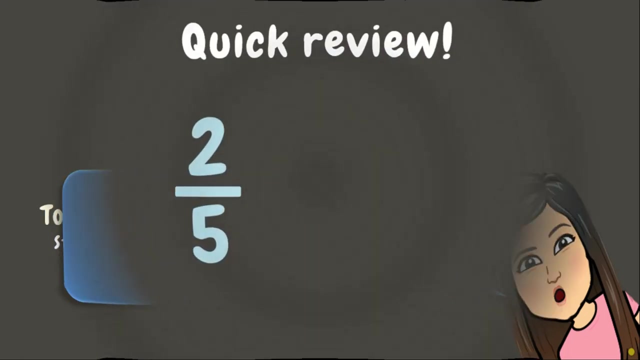 step is to get the reciprocal of the divisor or the second fraction. But how are we going to get the reciprocal of a fraction? Let's have a quick review. To get the reciprocal of a fraction, we just simply switch the positions of the numerator. 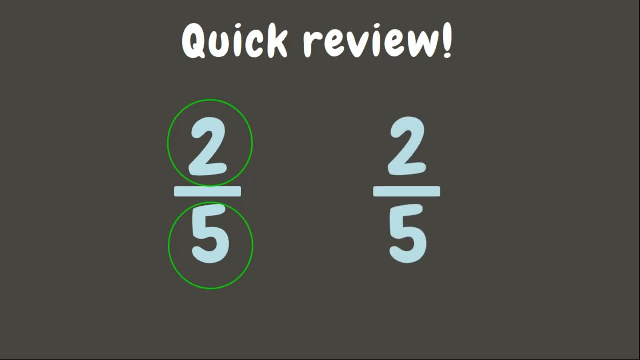 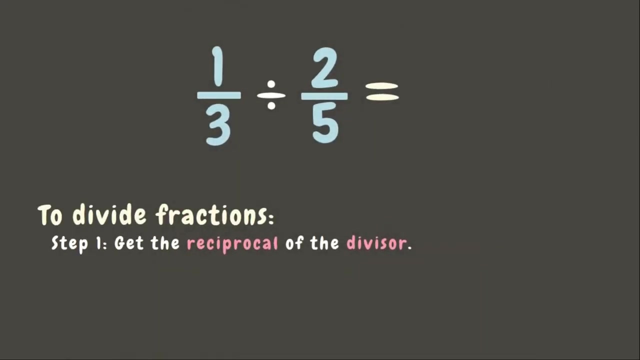 and the denominator There. Now the reciprocal of two-fifths is five halves. Now let us go back to our problem. Now let's get the reciprocal of the divisor two-fifths. There you go. The next step is we need to change the operation to: 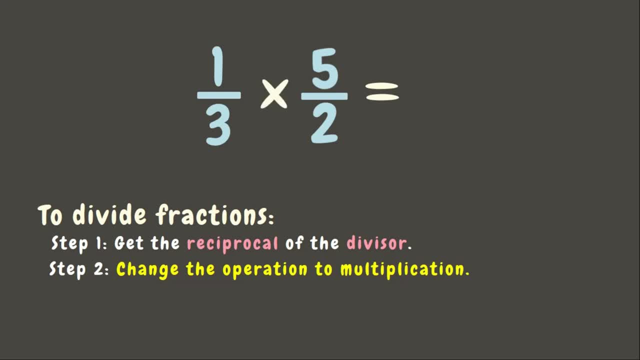 multiplication, And it's time to multiply the numerators and the denominators. One times five is five. Three times two is six. Since our answer is already in its simplest form, this is now our final answer. Now let's have more example. Let's. 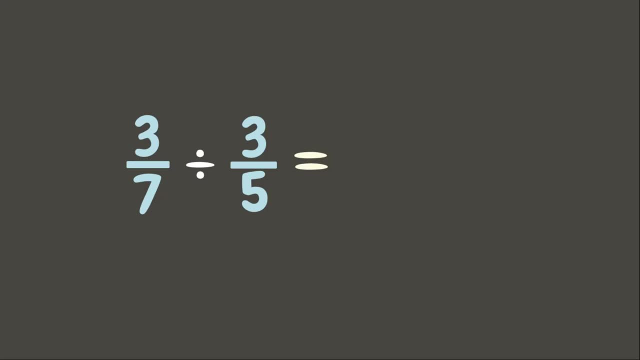 try three-sevenths divided by three-fifths Again. what is our first step? You are right, We need to get the reciprocal of the divisor three-fifths. Let us switch the numerator and the denominator There. Now let's change division into: 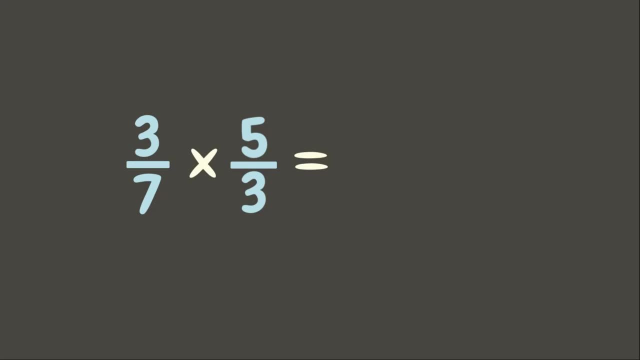 multiplication. Now let us multiply the numerators and denominators. Three times five is fifteen. Seven times three is twenty-one. Is this our final answer? No, not. yet We can divide fifteen and twenty-one by their greatest common factor, which is three. Fifteen divided by three is: 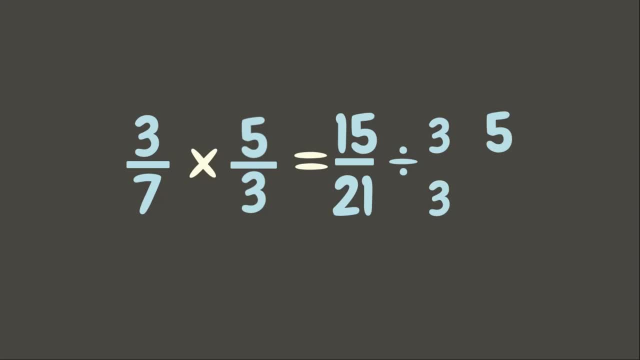 five Twenty-one divided by three is seven. Now, this is our final answer. Now let's have three- його's term. now Let's turn back to the licensure and the numerator. We have to draw a three-zeit differential to solve our experiment. But we'll see how accurate this, yours, is, as 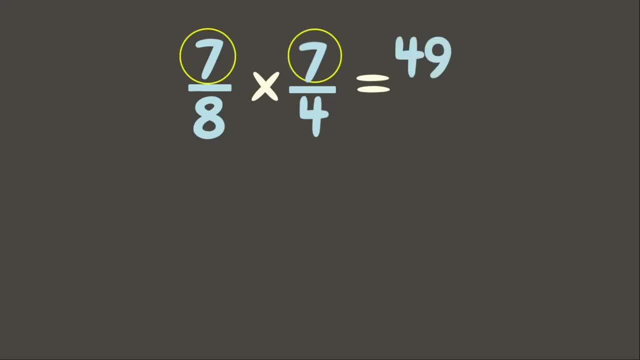 the calculator shows us: Okay, Maybe you have some allied grammar south on either of these answers Again. Oh boy, Oh well. eight times four is 32. since our answer is an improper fraction, we need to change this into a mixed number: 49 divided by 32. 1, 1 times 32 is 32, 49. 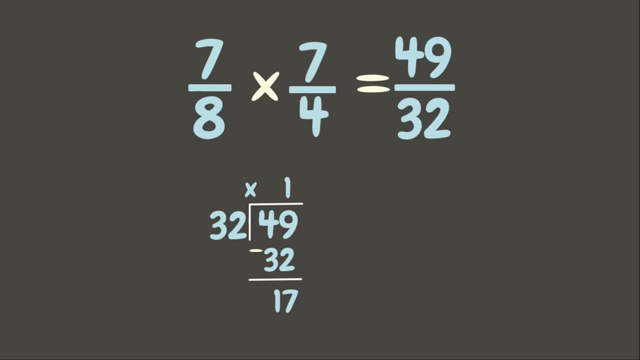 minus 32 is 17. now our answer is 1 and 17 out of 32. next one: how are we going to divide a fraction by a whole number? this is just the same on how we multiply a fraction to a whole number. first is we put one. 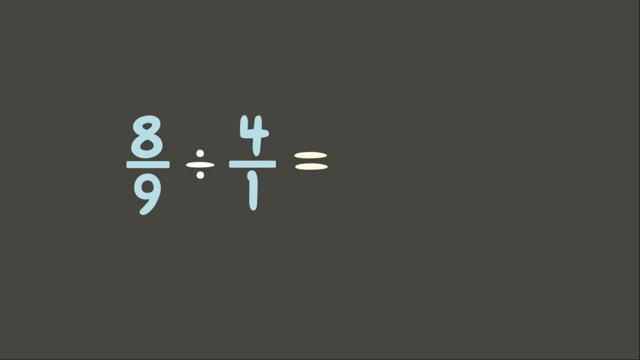 as the denominator of the whole number, and then let us get the reciprocal of the divisor there. now change the vision into multiplication. let us multiply 8 times 1 is 8. nine times four is 36. let us simplify our answer: 8 and 36 can be. 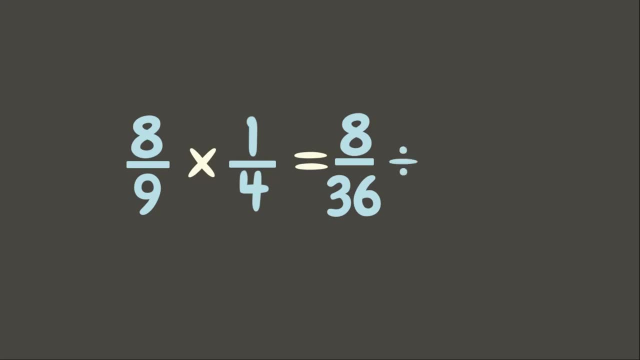 divided by the common factor four, eight. divided by four is two above 36. divided by four is two above 36. divided by four is two above 36. divided by four is two. edit: four is nine. now two ninths is our final answer. now, how are we going to divide a? 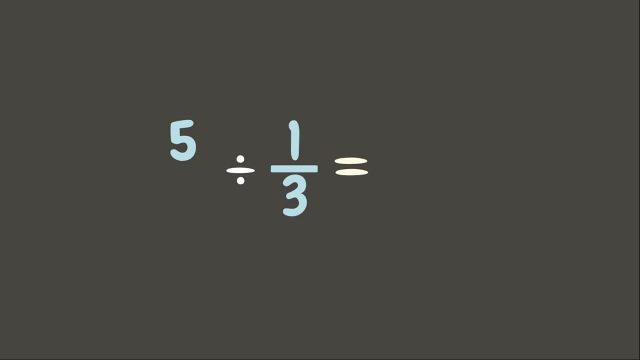 whole number by a fraction. let us put one as the denominator of the whole number. next, get the reciprocal of the divisor. change the vision into multiplication. let's multiply: 5 times 3 is 15. 1 times 1 is 1. now let us simplify. 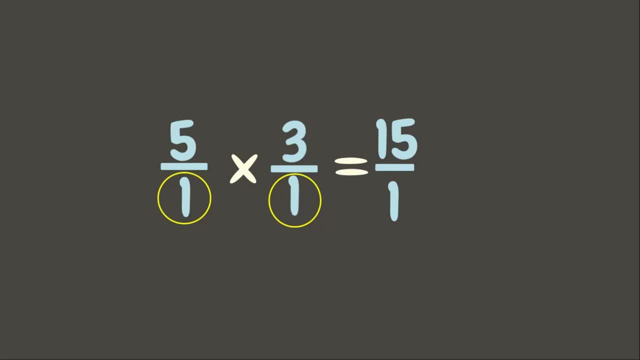 since the denominator of this fraction is 1, it will be equals to 15, because 15 divided by 1 is 50. now how are we going to divide mixed numbers? first, change the mixed numbers into improper fractions. 2 times 2 is 4 plus 1 is.